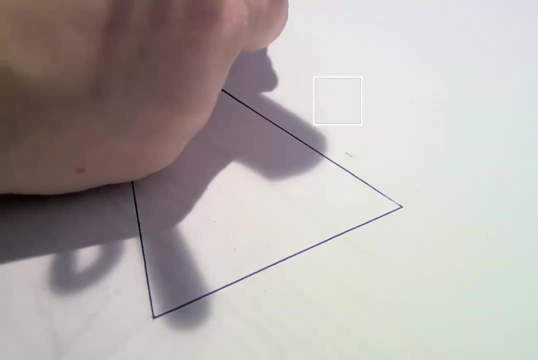 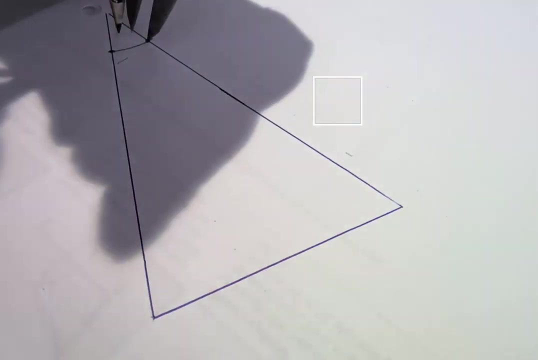 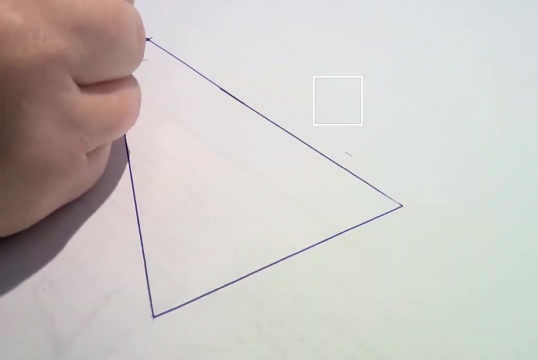 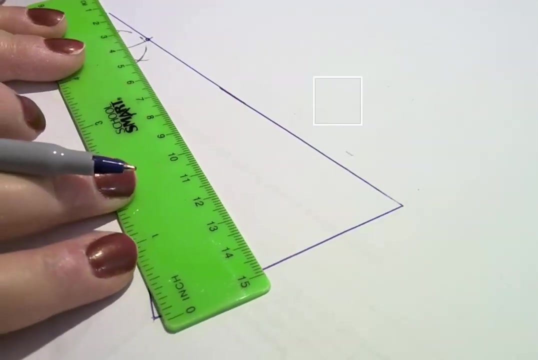 do the football And the football is going to actually be inside the angle here, So we end up with a little football in the middle here And the better we do, the better we get And we will be able to see in the end how we did. 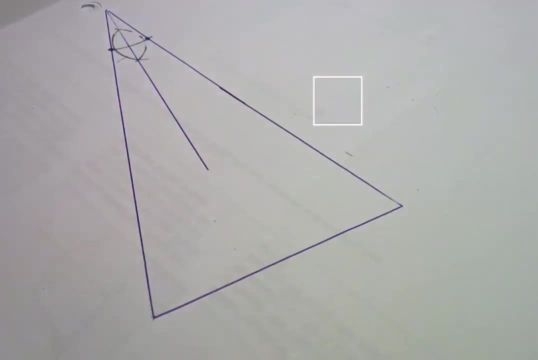 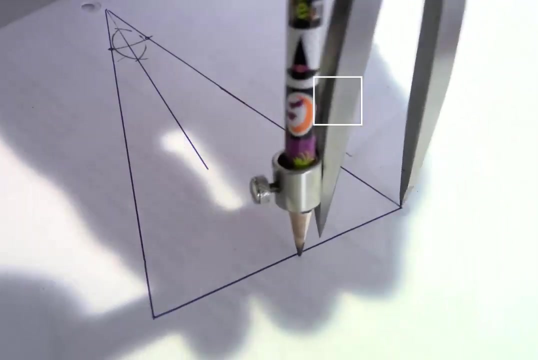 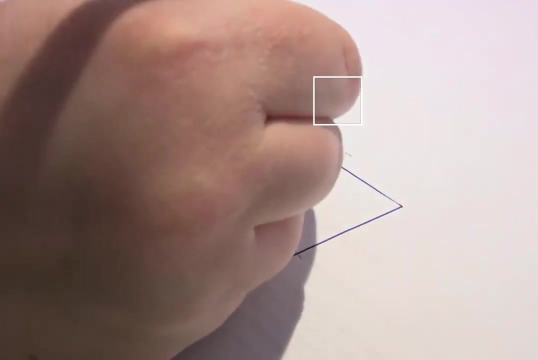 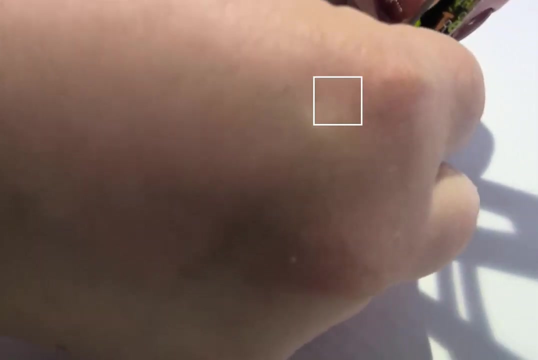 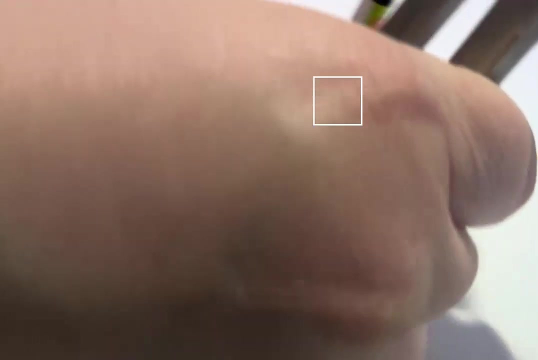 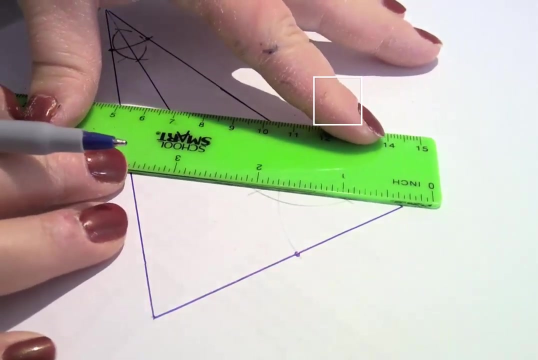 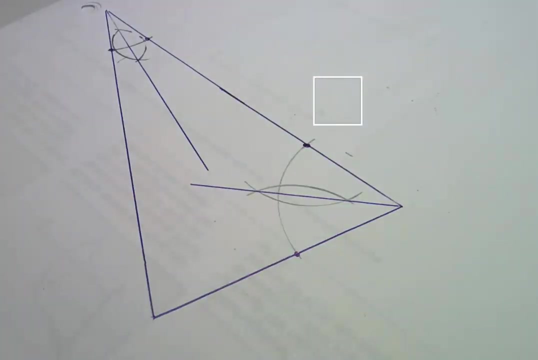 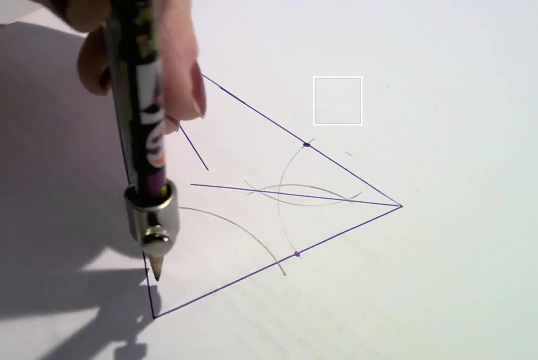 One angle, bisector, Make it a little bit bigger. And the next angle: we need to hit it on both sides, Going in between here and here With a football. 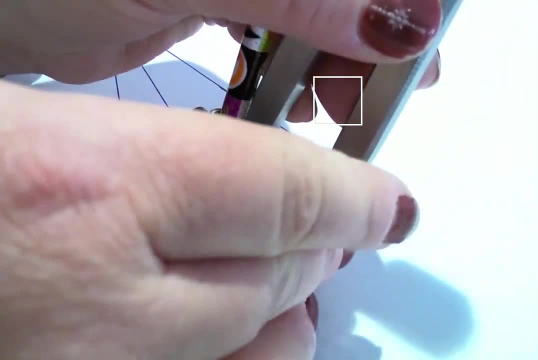 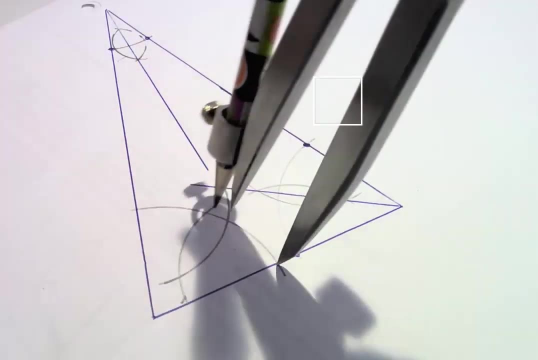 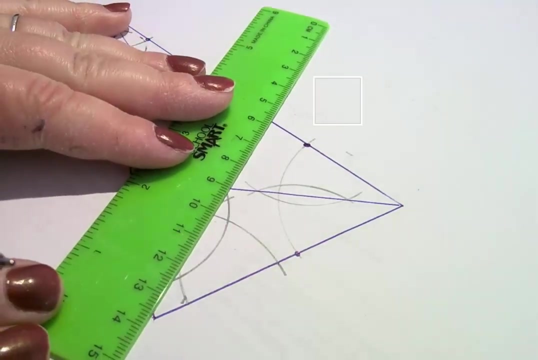 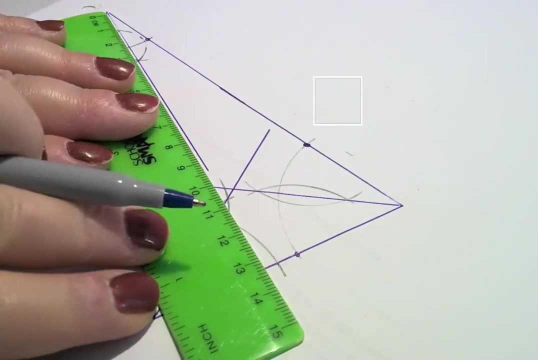 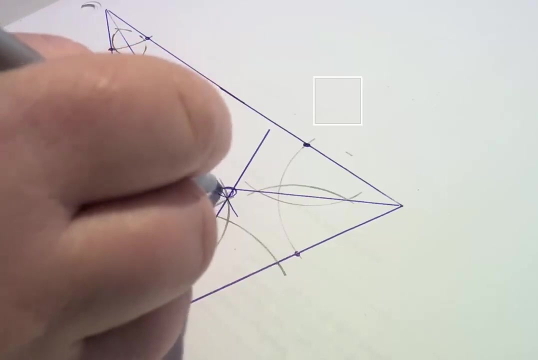 And if we extend all these angle bisectors, they should all hit at the same place. Uh oh, Not good. They're supposed to all line up at one point. I'm going to make it a giant point right there. 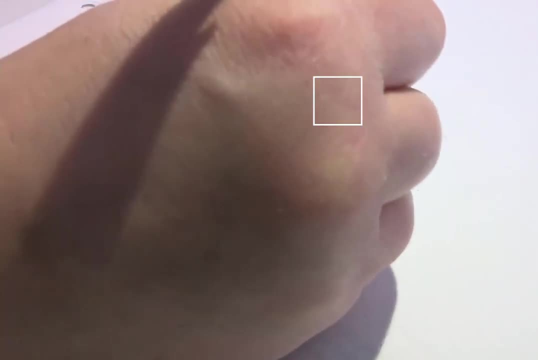 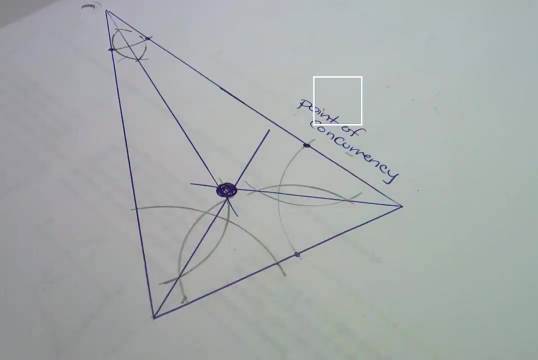 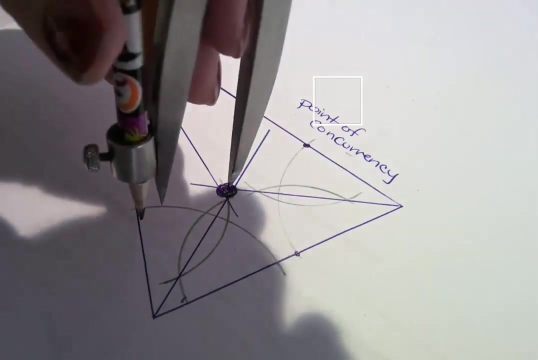 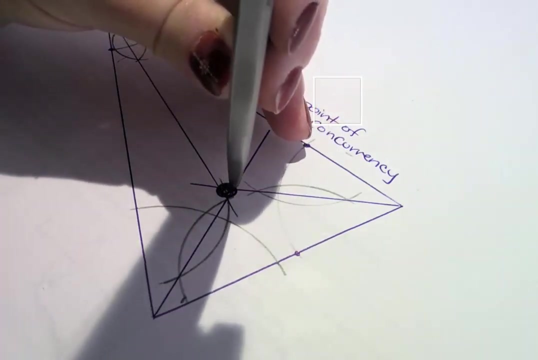 We call that point the point of concurrency. The cool thing about angle bisectors is that if you put your compass on this point and stretch it so that it just grazes one side, it should graze all three sides as well. So if I stretch this compass to hit here, on this side,